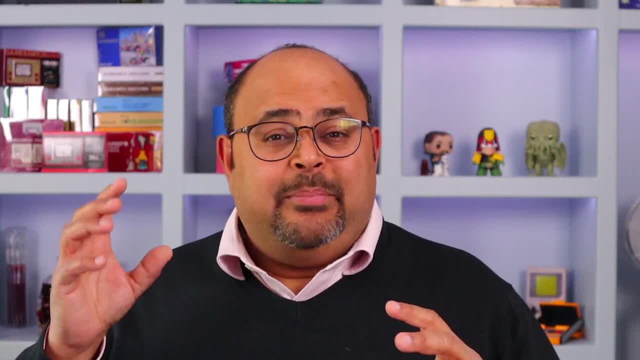 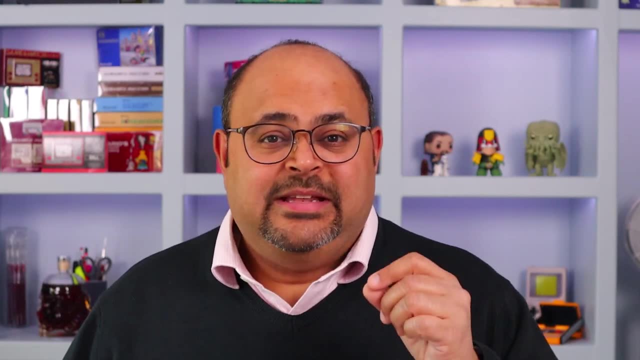 overwhelm what you start with because you're trying to keep it simple. well then, perhaps that would be the perfect candidate to put into an expansion later on. Now I want to stress that when I say keep it simple, I don't necessarily mean the game has to be simplistic. You can have 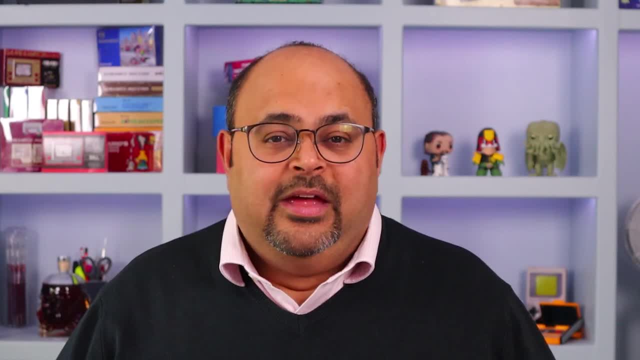 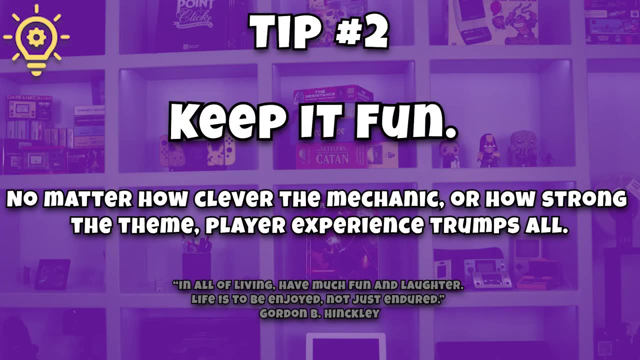 quite complex games. but you can have quite complex games and you can have quite complex games and you can have quite complex games at the end of your development. But to start with, start with a base mechanic, start with a core game. When I started this little journey, I was under the 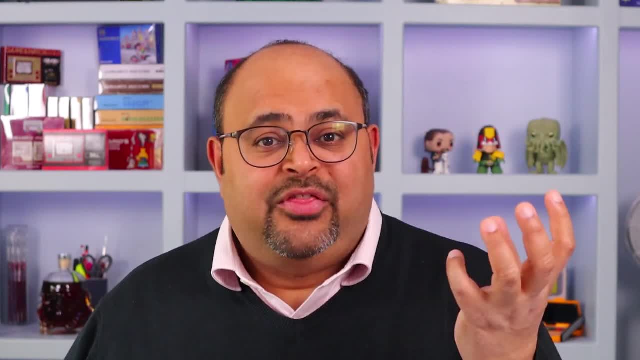 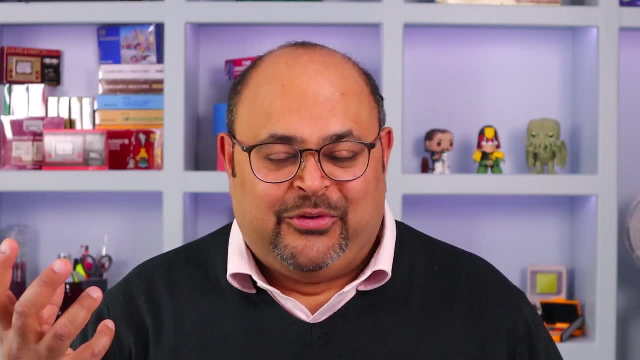 assumption that all ideas were either centered around building a theme on a really clever mechanic you had thought of, or building mechanics around a really clever theme that you had thought of. Well, the reality was that actually both are important, And I think that's what I'm going to. 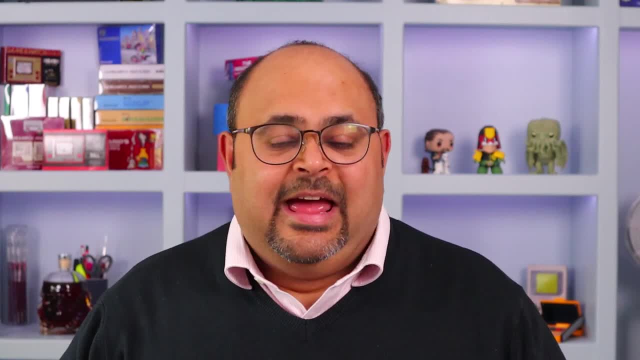 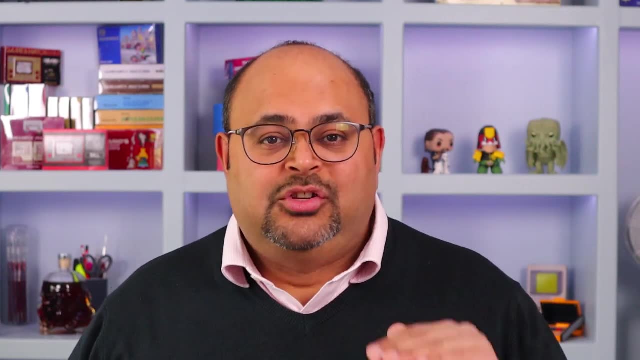 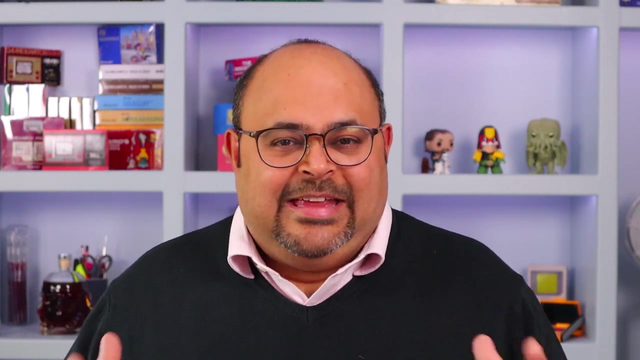 talk about in this video, But neither are as important as the player experience. What is it that you want your players to feel Now, above everything? it's got to be fun. For it to be a game, you have to have fun. It seems obvious, but sometimes we forget that because we're really 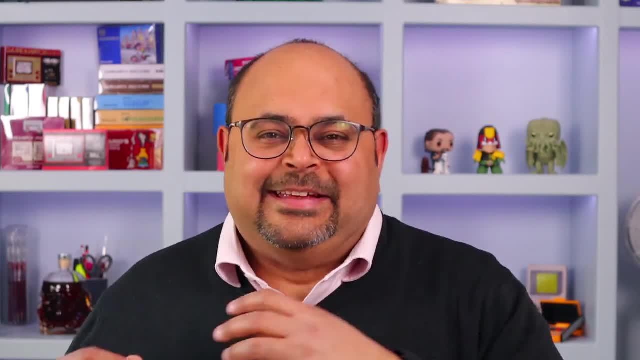 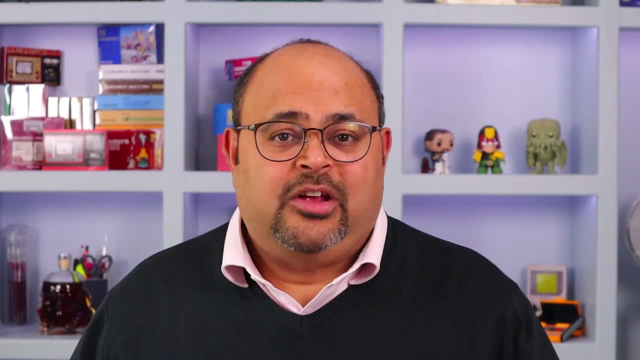 caught up in our theme or our mechanics. more often it's mechanics. Fun for you may be different for fun for me. A game of Snap is fun- if I'm playing with my little nephew, for example- But it's only fun for a few rounds and even then he'll get bored. Imagine that same fun game. 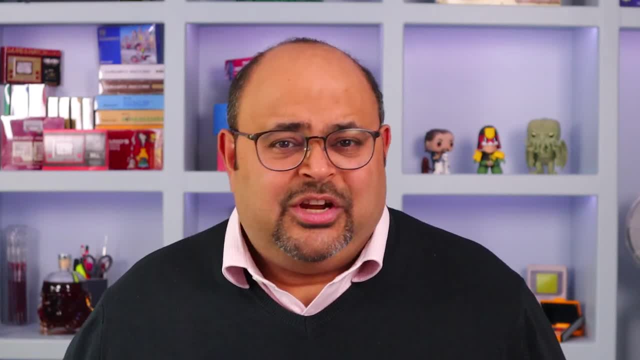 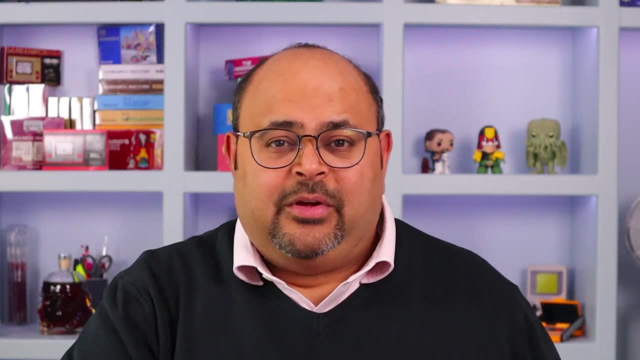 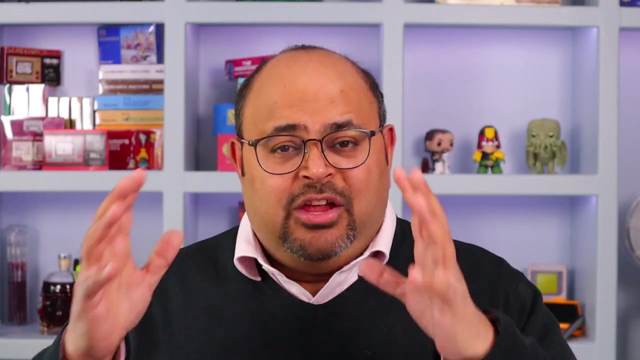 being played for three hours with a grandmaster's chess champion. It's fun for no one. It's very dull. Similarly, a very complex game may not be fun for someone of a very young age or someone who's looking for something that's much more random to play. You need to think of what the 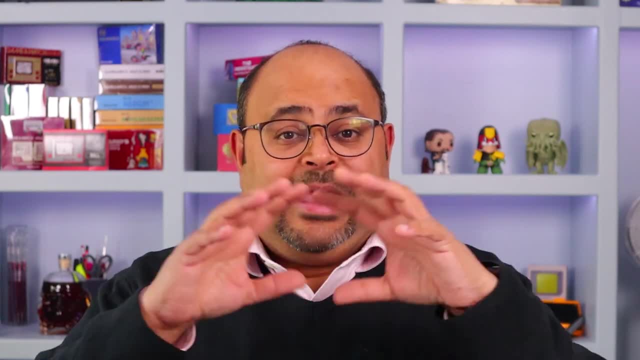 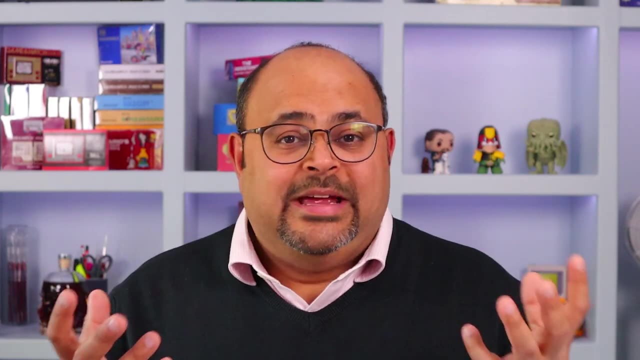 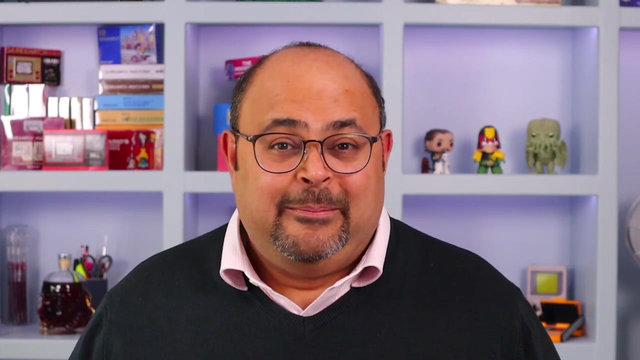 end result's going to be who you're targeting for and ensure that that player experience is felt through your mechanics. Remember, mechanics and theme can all be adjusted to find and fit that game or experience. Thinking back to Zintis and his cave paintings game, he had an idea of what he wanted his players to feel. 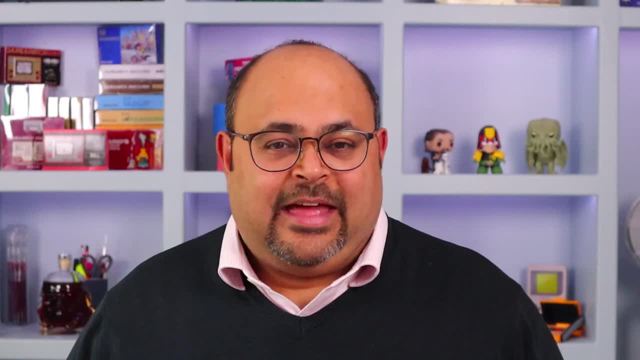 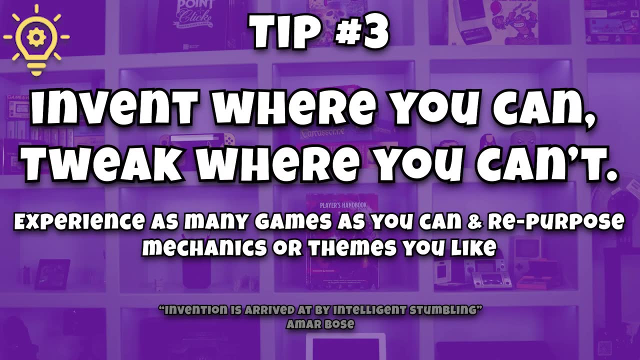 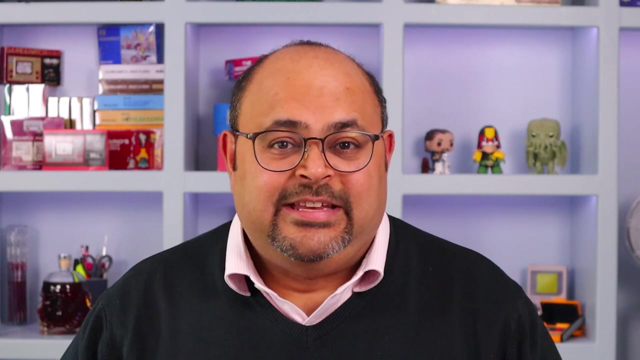 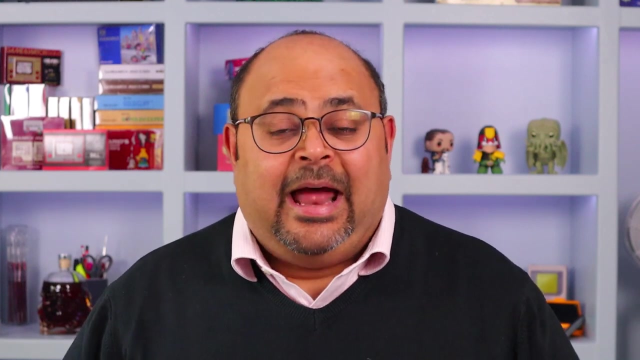 and then adjusted to mechanics to be able to get that player experience through in his game. Now I'm paraphrasing, but Mal had said to me that you should not be afraid of using what's out there And adjusting it to your own ends. Again, 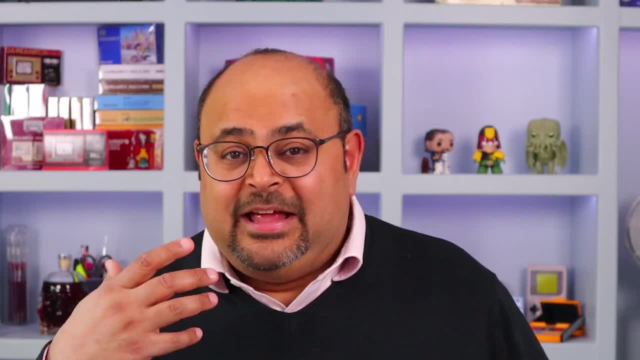 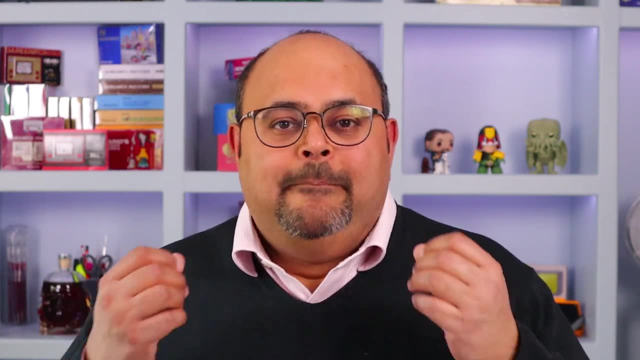 that was iterated by others that I spoke with, And every time I read something in a forum or I go through an interview on paper, I read the same things. Don't be afraid to use some of the ideas that already exist, but tweak them and make them your own. 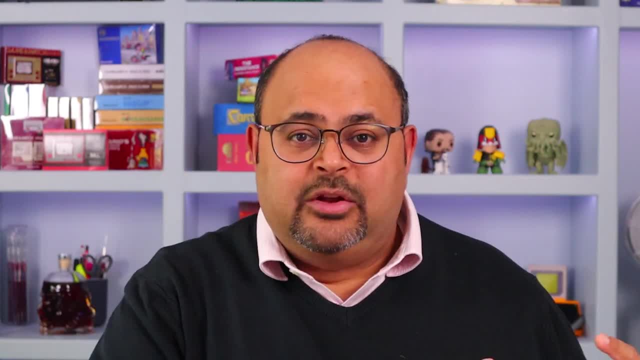 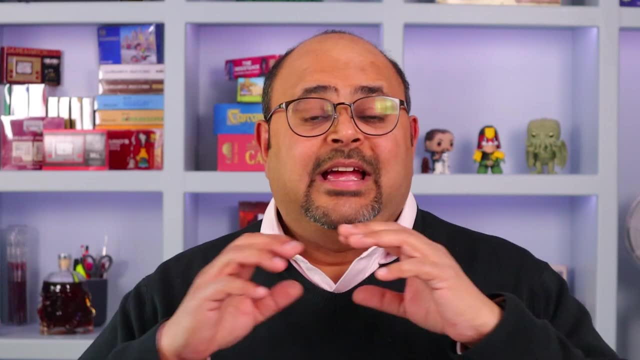 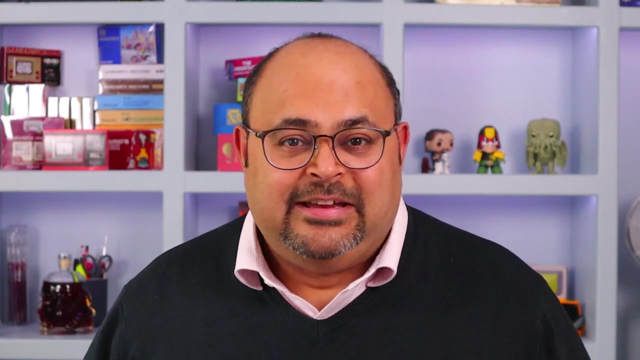 Maybe you've got a great setting and you've seen a really good mechanic. There's nothing wrong with taking the mechanic, tweaking it and adjusting it to fit into your theme, creating a completely different player experience and really the beginnings of a new game. Don't be afraid to. 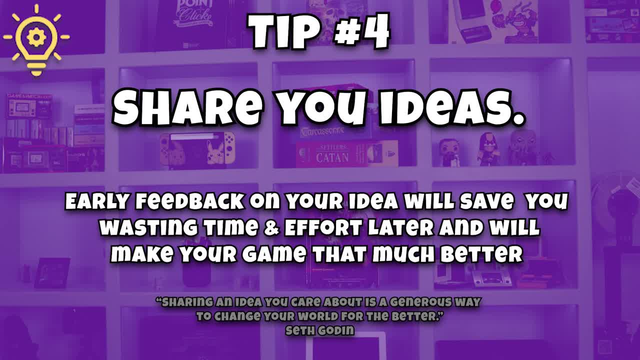 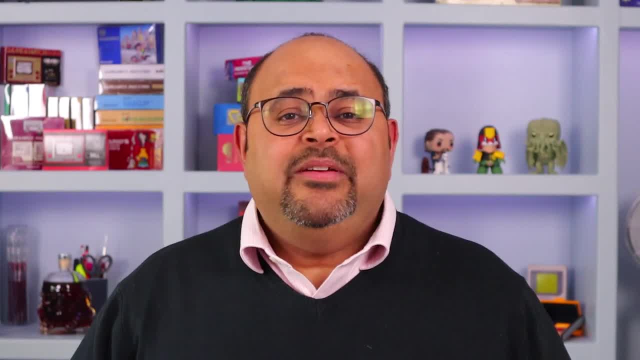 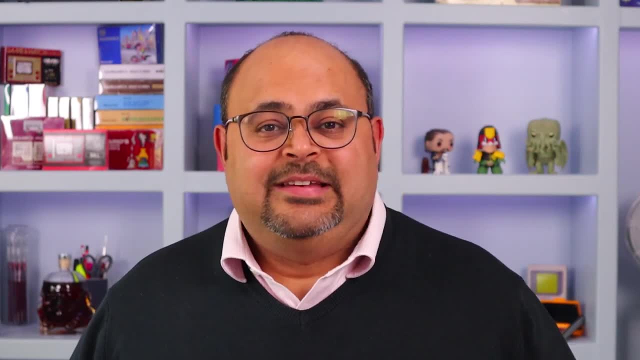 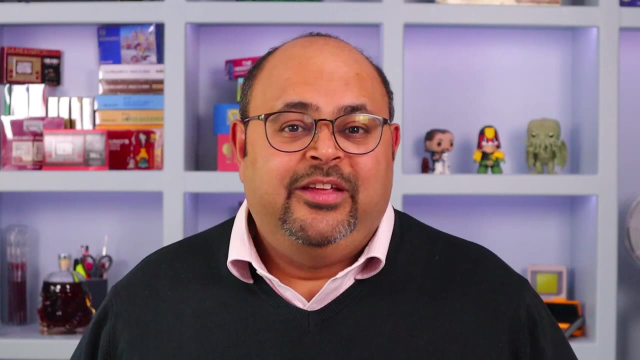 reuse what's out there. Obviously, we are going to have to test your ideas. But even before you begin that process of building a prototype or a set of test components, one of the top ways of validating whether you have even the beginnings of a good game is to share the idea And sharing. 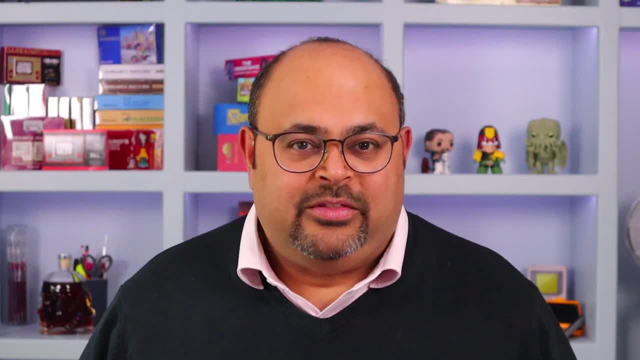 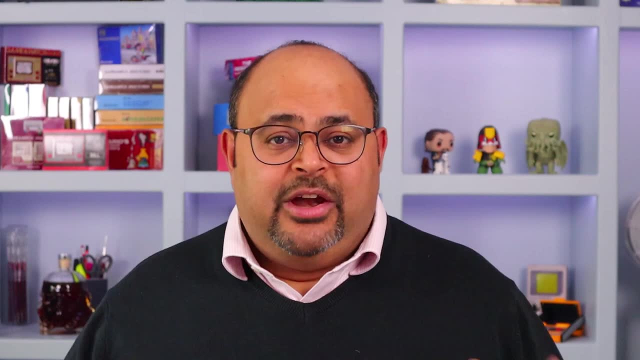 the idea is one of the things I had a big problem with and still have a big problem with, But from all of the developers I heard the same thing: Sharing your idea means you get more feedback on what is possible. The idea you have at the moment is really important And I think that's. 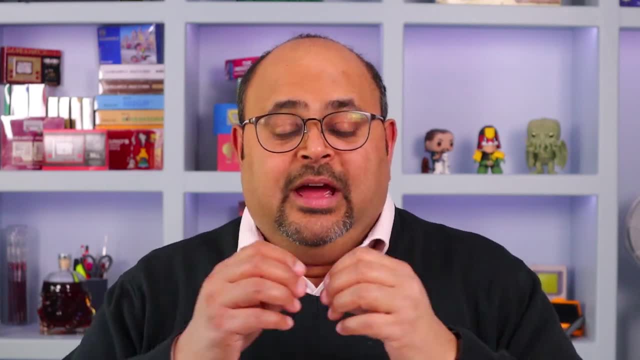 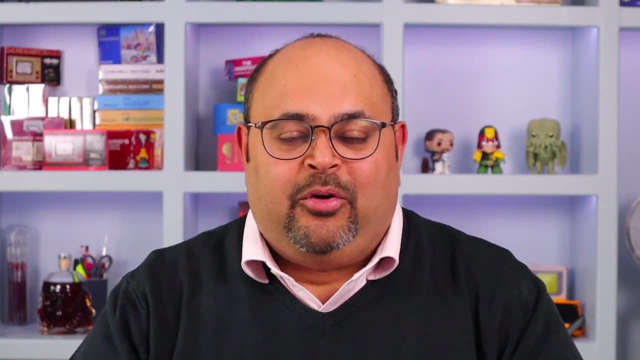 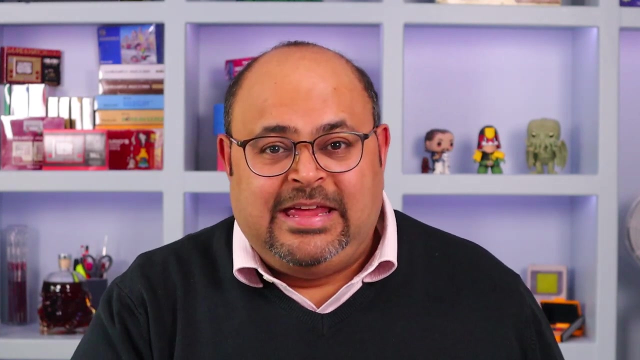 really a problem. It's a problem that needs a solution, And that solution will end up being your game. But right now you've got this wonderful idea that you want to put down onto paper or onto card and you don't know how Well, share it. Put it out there on Reddit or on BoardGameGeek or on. 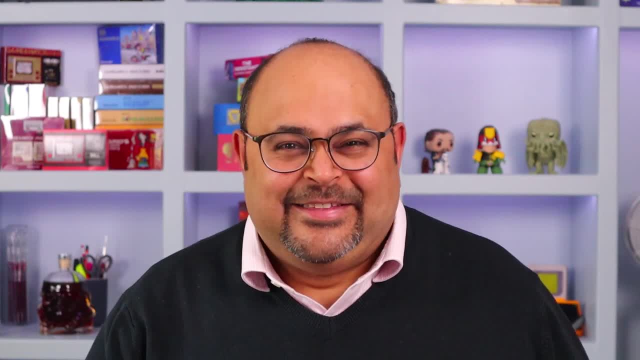 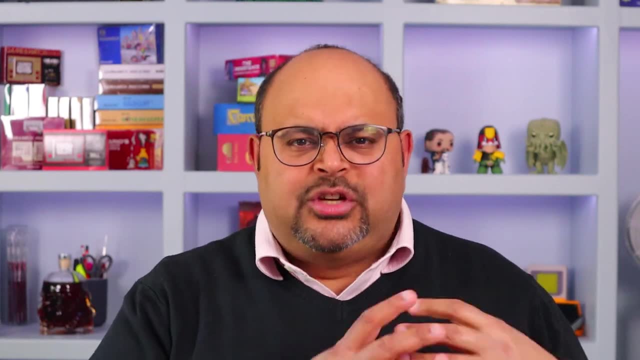 BoardGameAtlas or any one of the hundreds of outlets that exist on the web. now Have that conversation. You don't need to share the finer details if you don't want to, but share the general idea and get that feedback. What do people think? Does this seem like a good theme? Is this taboo? Is 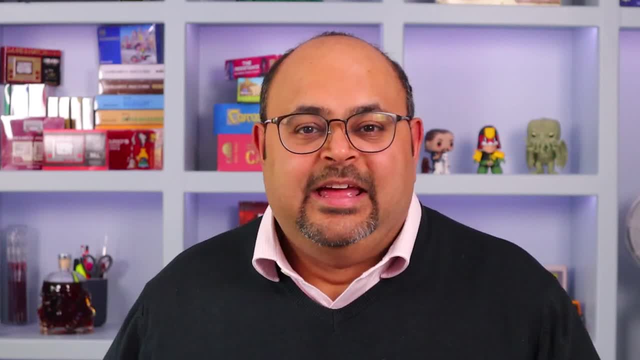 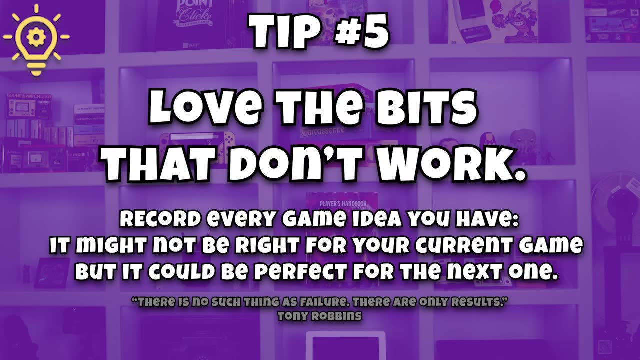 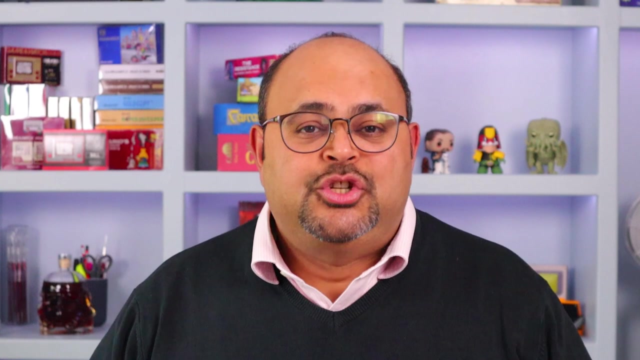 it something that you don't think is going to be thought of. Share the idea, Benefit from the wealth of knowledge that's out there And finally, you're going to fail. Some of those ideas are just not going to fit in the theme or the player experience you're looking for. Some of those. 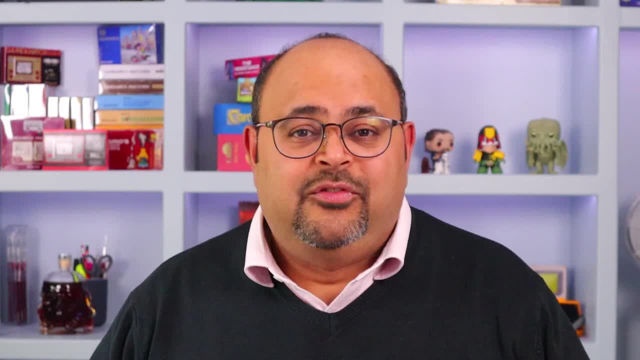 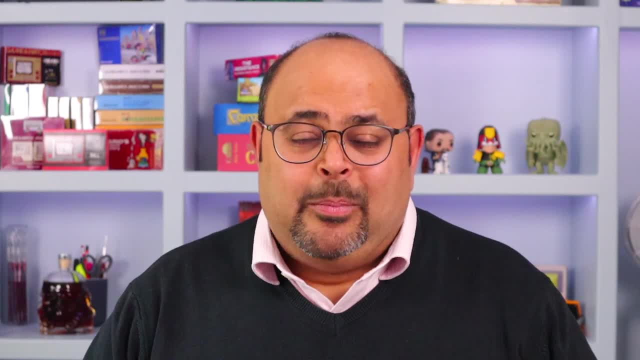 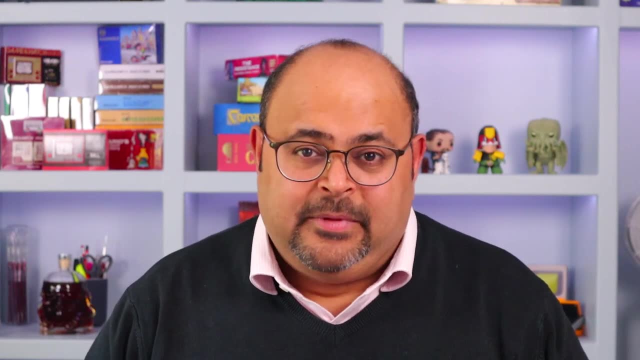 going to fail, You're going to fail, You're going to fail, You're going to fail. And sometimes, no matter what you do, your player mechanics, your game experience- it's just not working. Your experience is just not fun, And that's okay. Be aware that, especially if you go down the 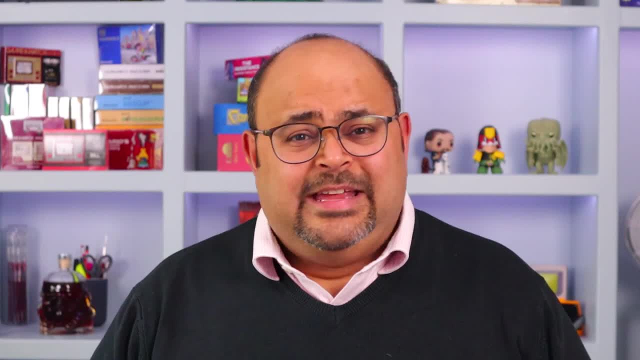 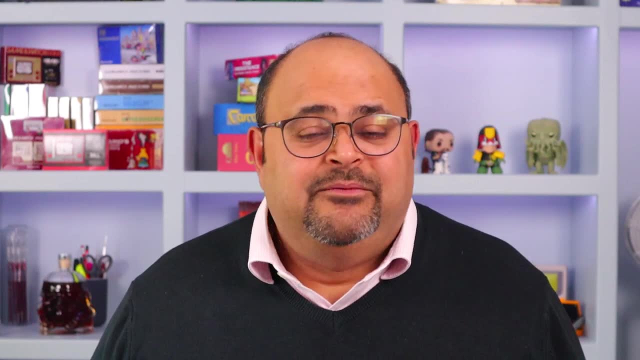 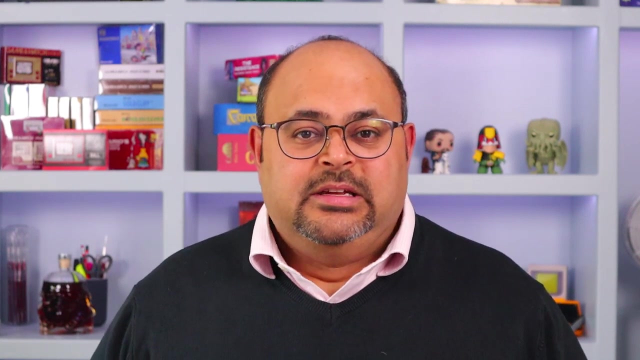 publishing route where you get a publisher on board. your idea is going to be changed. Your initial thoughts are going to be completely transformed. Your artwork that you may have envisaged will change. All of that is okay. none of that is a bad thing, and there are no bad ideas. just record them down in your journal. 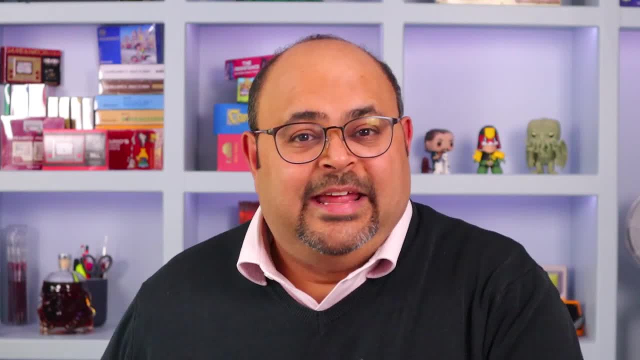 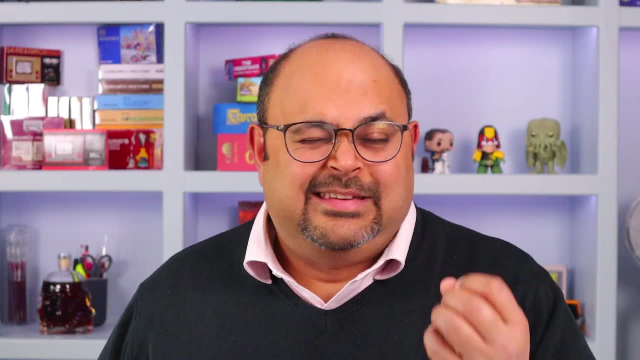 and use them in the next project, use them in the next game again. when i interviewed those guys, i heard the same stories. i heard the fact that they tried something. it didn't quite work, and then they were on a different project, a completely different game, and they were thinking about how to solve a. 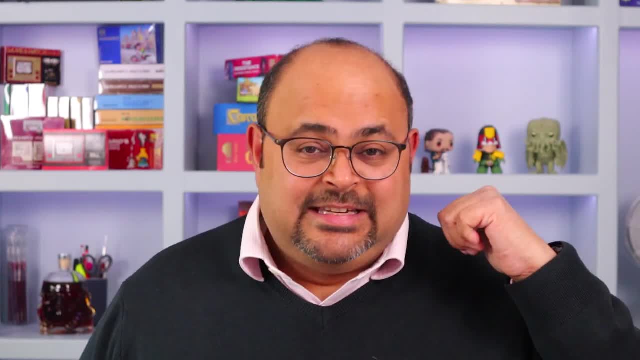 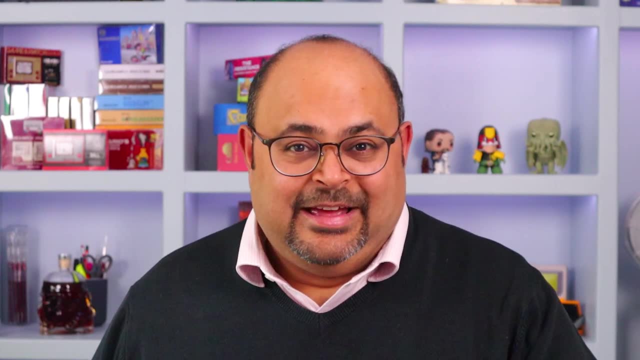 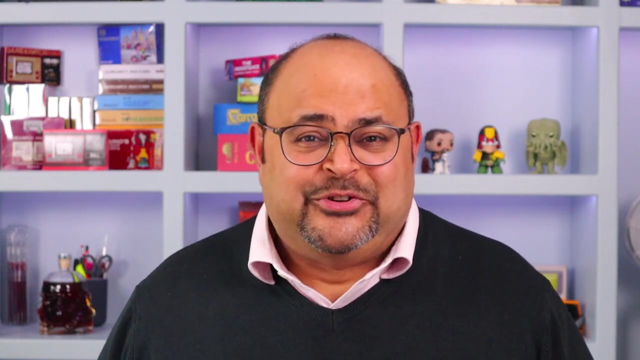 problem and, lo and behold, they had the solution. it was existed from a previous project or a previous game they'd worked on. there's nothing wrong in having a bit of failure. failure is how we measure success, as they say. oh god, i've ended on a cliche. i'm sorry, but it's true. well folks, i hope you. 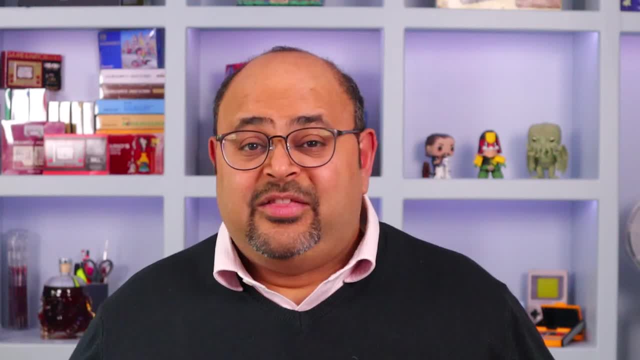 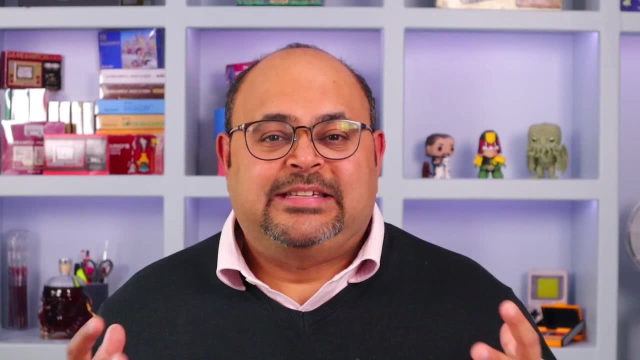 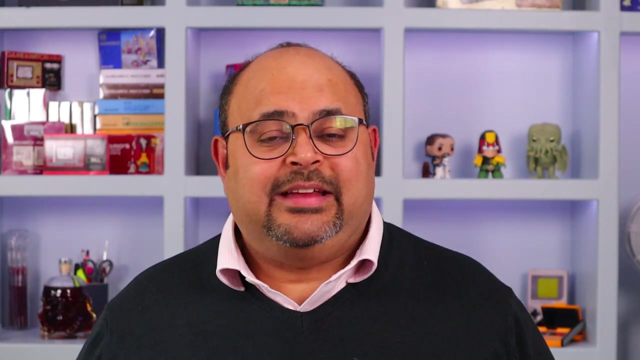 found that useful. i know i did. i want to take time out again to say thank you to the five individuals and a multitude of people on reddit, especially for helping me out and understanding exactly what it takes to you to shape a good game idea. now that i've done that, i think i'm ready to move on to the next stage.